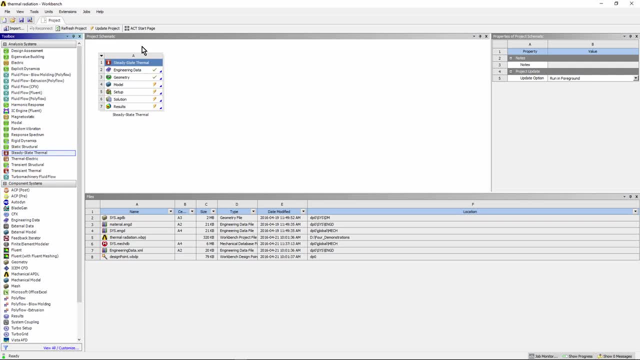 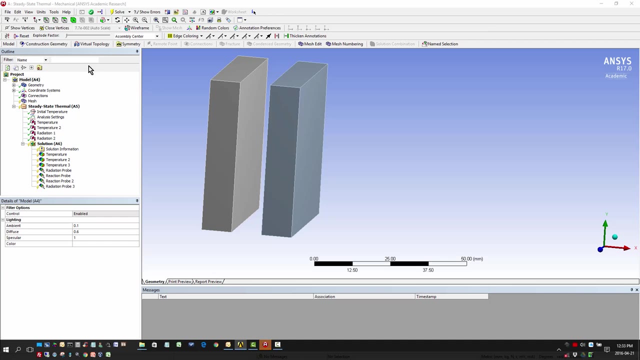 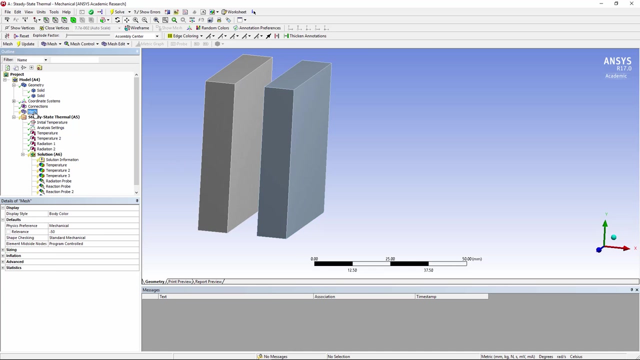 it out into the project schematic area. We've imported the geometry, which is of the two plates, and now we can click on model right-click and edit using Workbench Mechanical. Here's the imported geometry. We have two solids and they're facing each other We're going to use 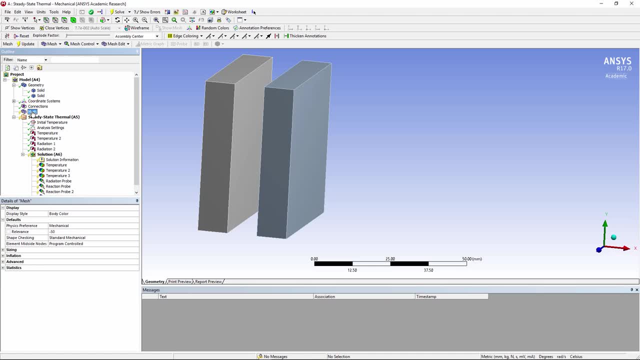 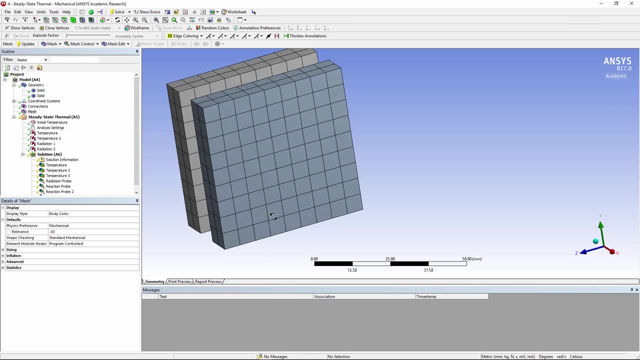 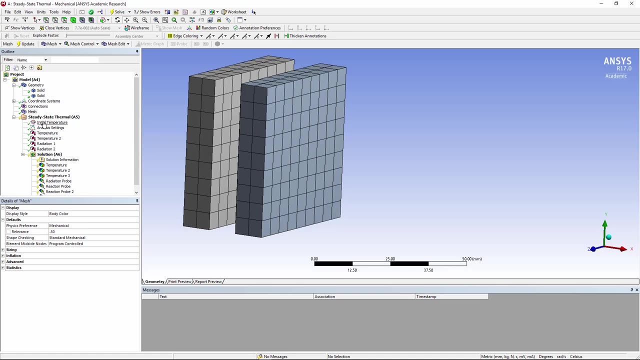 simple meshing. with the relevance turned down, Let's right-click and generate a mesh Here. now is a simple mesh and since it's a thermal model, there'll be thermal elements. For an initial test, let's take a look at the temperature. Let's assume room temperature. That's the default. 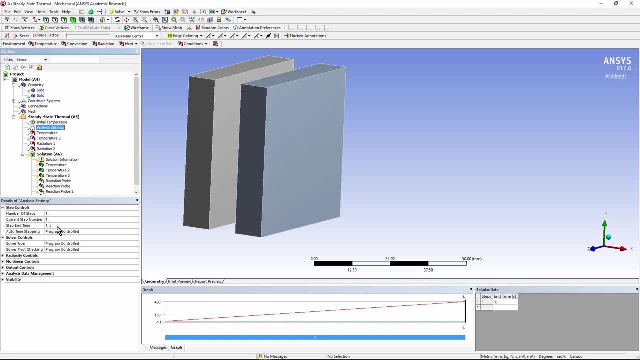 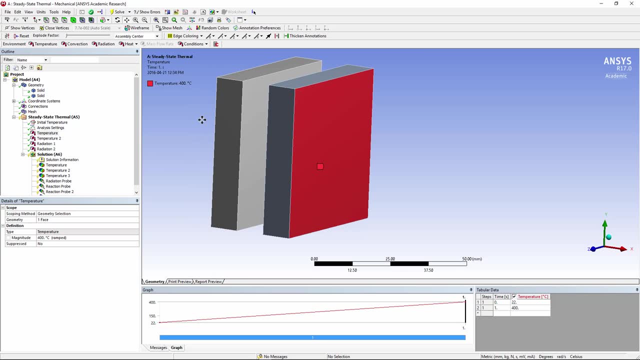 In our analysis settings. we have just one load step and everything is at default For our temperature loads. on the right-hand side you can see that we have 400 degrees Celsius. On the far left-hand side, we're at room temperature 22 degrees Celsius. This is going to create quite 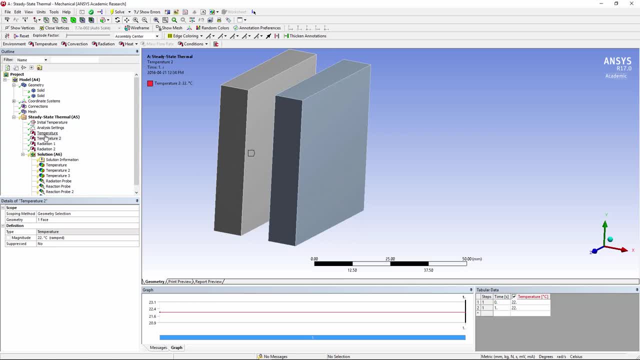 different temperatures in these two blocks. Let's take a look at the temperature on the left-hand side. Now. our radiation boundary condition could have been set to both of these interfaces that look at each other, but we're breaking them out here into one on the left side and one on the 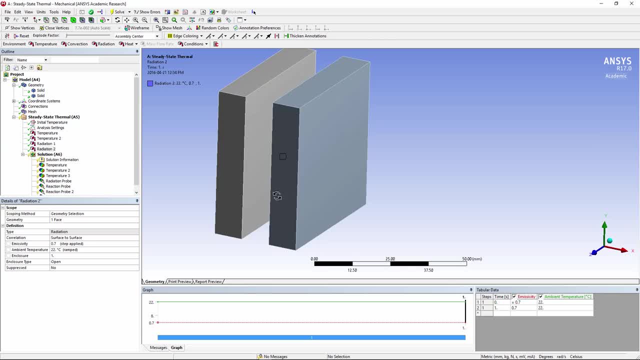 right side so that we can isolate the reactions on those faces. Now, on that left side we're assuming ambient temperature, That's a free space at 22 Celsius, so it will radiate out of these gaps to the external space. Now let's take a look at the temperature on the left-hand side. This is going to: 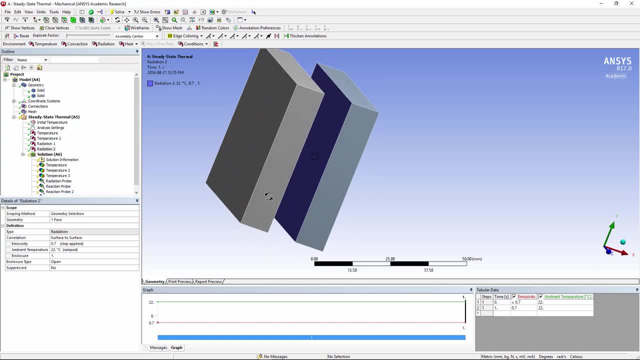 radiate out of this area And on the other body again. emissivity 0.7,. ambient temperature of free space is 22.. Note that it has enclosure number one. And if I go back and look at the other face, 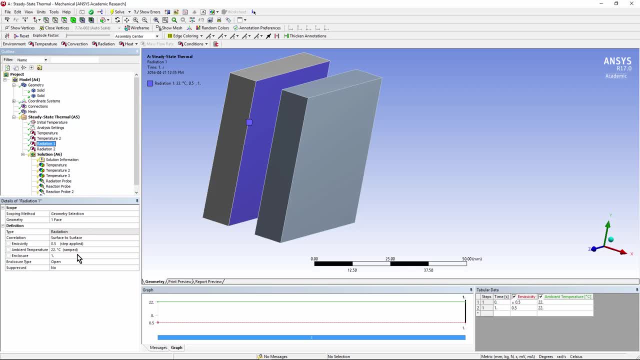 it also has been given enclosure number one With matching enclosure numbers. they will radiate to each other, Otherwise they would ignore each other. Our enclosure type has been set to open. If I set it to perfect, it's not going to radiate to free space and I will not be given the 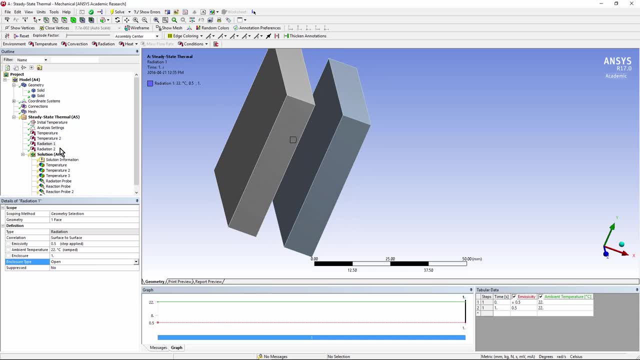 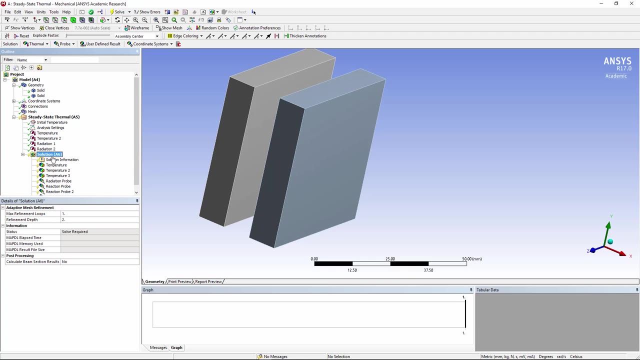 chance to put in an ambient temperature. Similarly, on the other side it's an open enclosure and I do have an ambient temperature. We're ready to solve this relatively simple radiation heat transfer problem, So I'll go to the solution branch, right-click and solve. 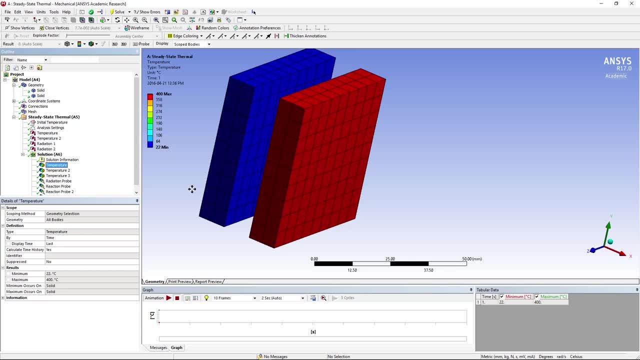 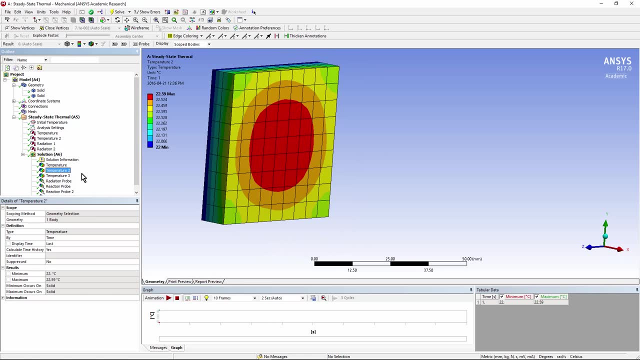 Here we see the resulting temperatures. Now the two blocks are at a nearly constant temperature. I've inserted one object. looking at the left block and you can see it goes just a little bit above the 22 degrees that was imposed on the left side And in the right-hand block. 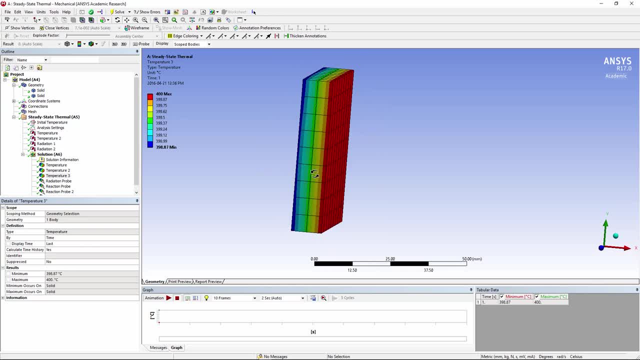 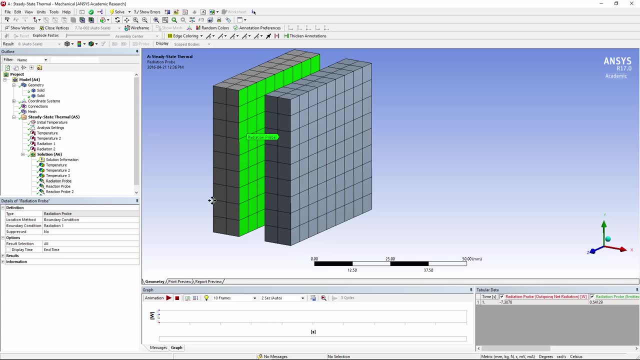 you can see that it does not go down very far from the 400 degrees that were imposed. If I put a probe on the left-hand face and open up results, I'll see that my outgoing net radiation is minus seven watts. Now if it was outgoing, it would have a positive sign because there's heat actually. 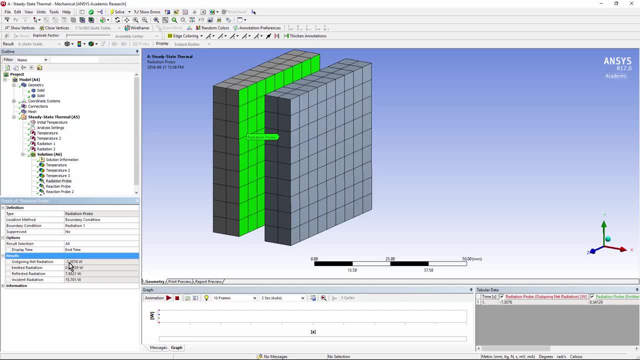 transferring in, We see the minus sign, so it's receiving a little over seven watts. The emitted radiation, because it's slightly warmer than free space, is just over half a watt. The reflected radiation, because the emissivity is not one, is 7.8 watts, while the incident what's coming in? 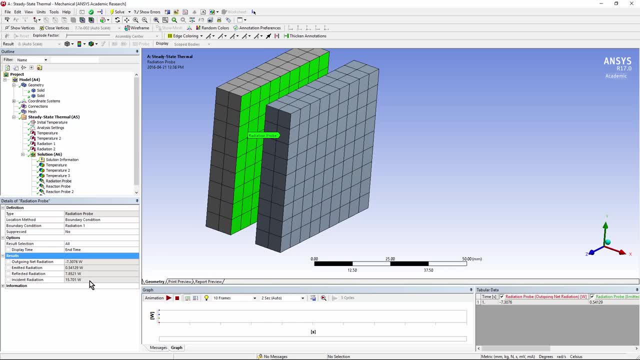 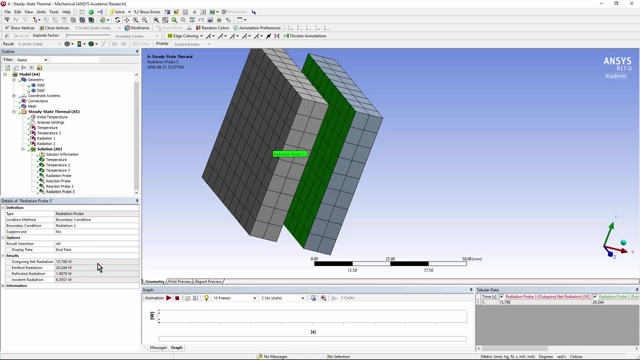 from the right-hand body is 15.. So some of the incident radiation is emitted. You can see the net. outgoing has a minus sign, so it's absorbing heat. We look at the other radiation probe. It's on the right-hand side and it's outputting 15.796 watts. That's the net. It's actually emitted as 20. A. 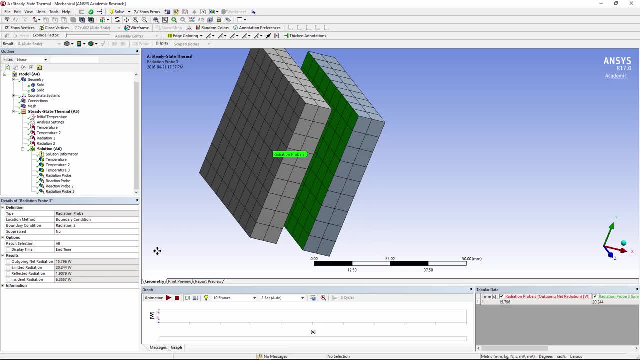 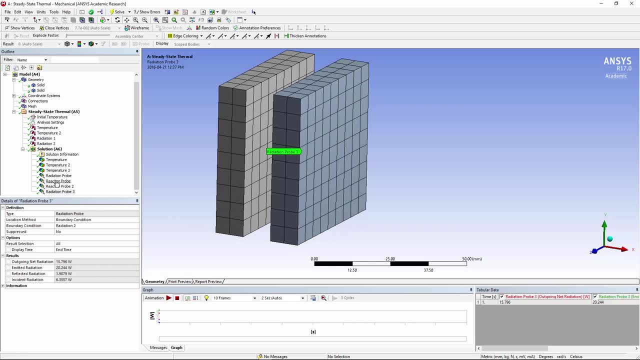 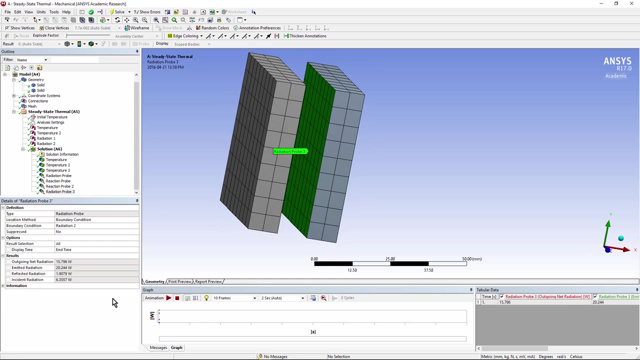 little bit is reflected. It's receiving some incident radiation of six point something watts. If I look at my reaction on the hot side, the right side, we're pumping in 15.796 watts. If I go back and look at my radiation probe, here there's the 15.796 watts, The same as we're putting. 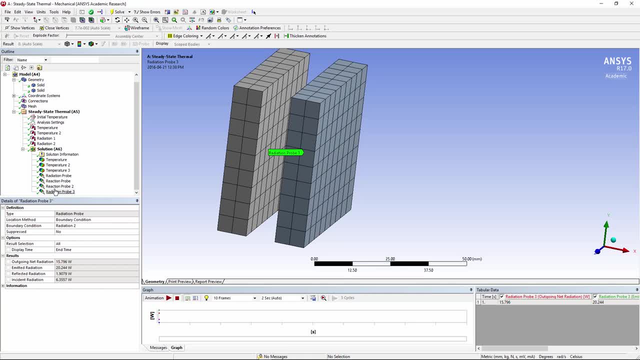 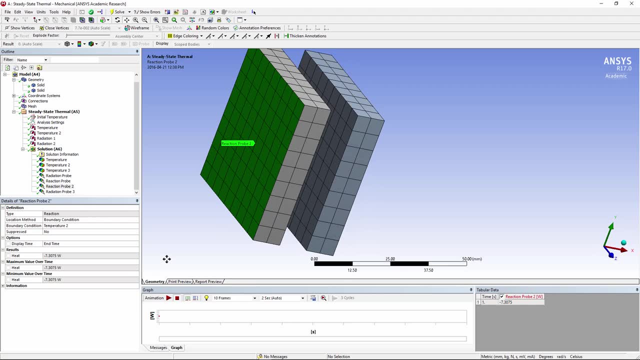 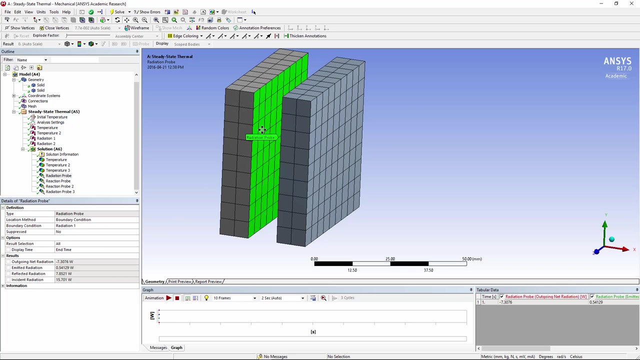 in on the right side. If I look at my reaction on the left side, where I'm holding it at 22, notice that it's withdrawing seven point three something watts And that is the minus seven point three watts, the net radiation that's coming in. So we're getting some. 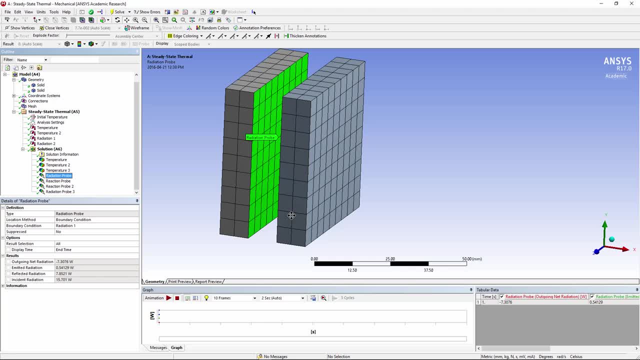 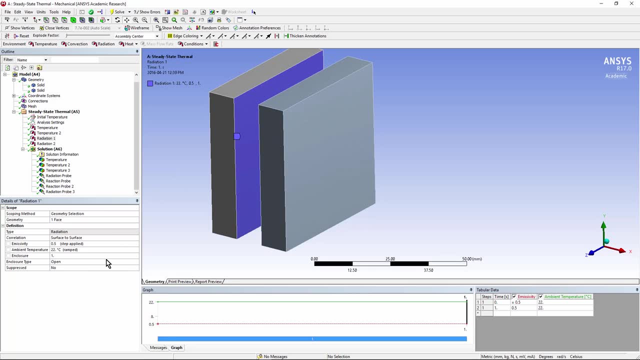 matching going on there. One final thing that's of interest is to go back to the first of these radiation inputs and see what would happen if we gave it an emissivity that was extremely low. Suppose we had it plated with polished gold. The emissivity might be as small as point zero two, and I'll enter and that'll change the amount of. 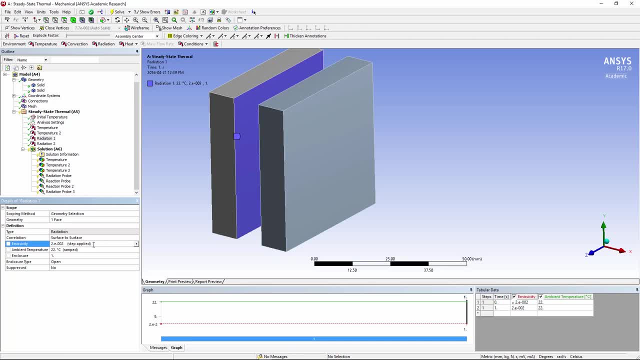 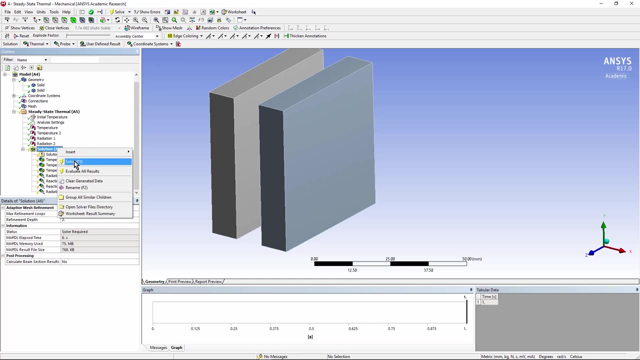 radiation heat transfer that's taking place. You might note that space vehicles sometimes have gold foil on them. It's being used because of the very low emissivity value in radiation heat transfer. Let's go and solve again Now. the temperatures are still at the two extremes. 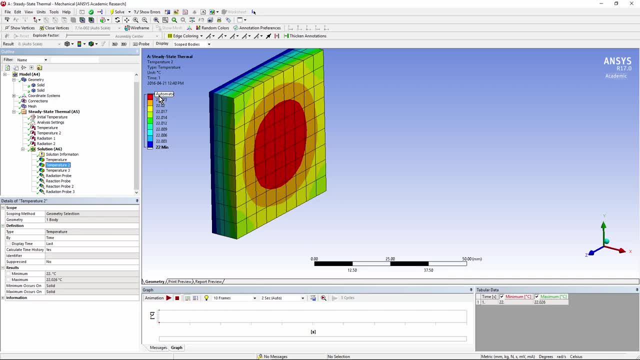 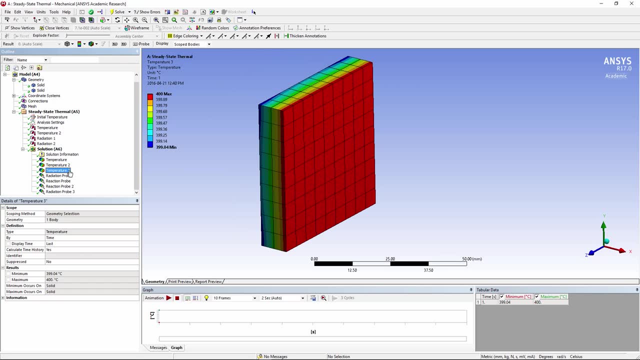 If we look at the left-hand body, it doesn't get quite as warm now, just up to twenty two point zero two six. The temperature on the right is similar to what we saw before. But look at the radiation probe for the left-hand side. 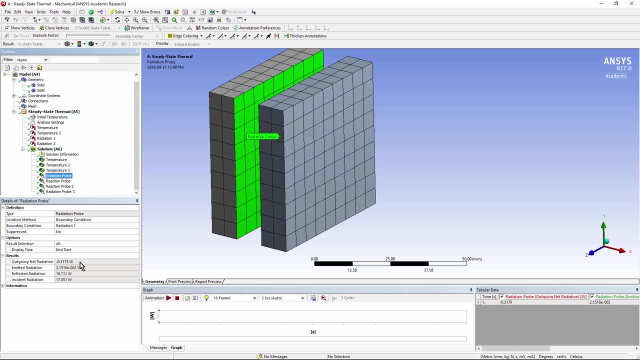 There's hardly any net radiation coming in because of that very low emissivity, and almost all of the incident radiation is being reflected. That's an interesting result and it shows how gold foil might protect something from being heated up, say by the light of the sun. 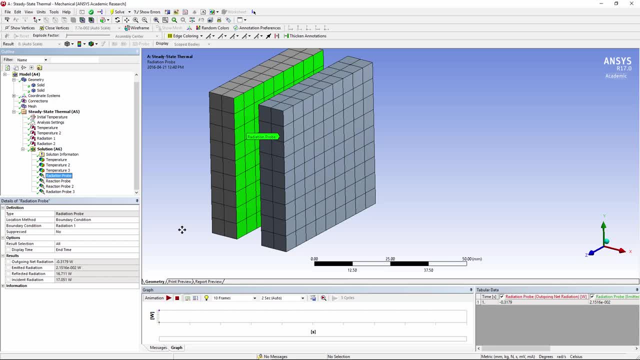 Thank you for joining me in this presentation on radiation heat transfer in Workbench Mechanical.